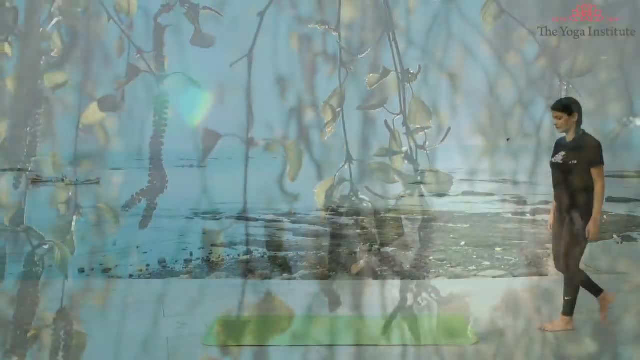 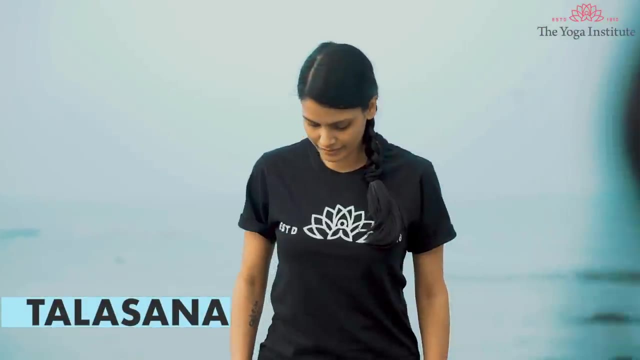 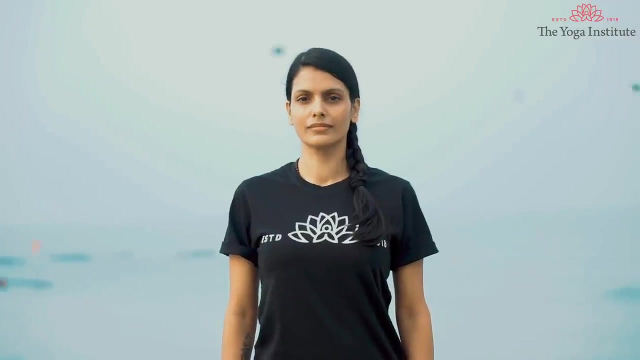 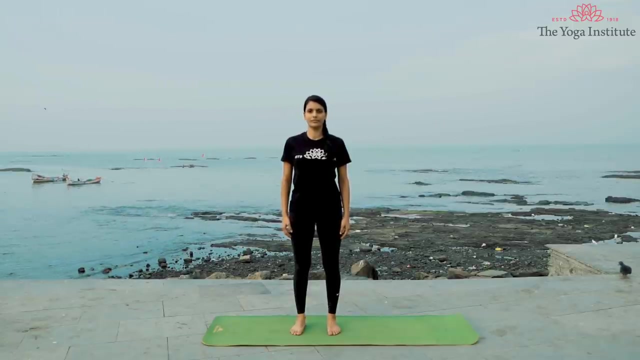 Let's get into the standing poses first. Talasana: Take one foot distance between your feet. Stand erect with your hands at your sides, Relax your shoulders and square your shoulders. Keep your chest expanded slightly and abdomen held firm. Now focus your gaze at one point in front of you. 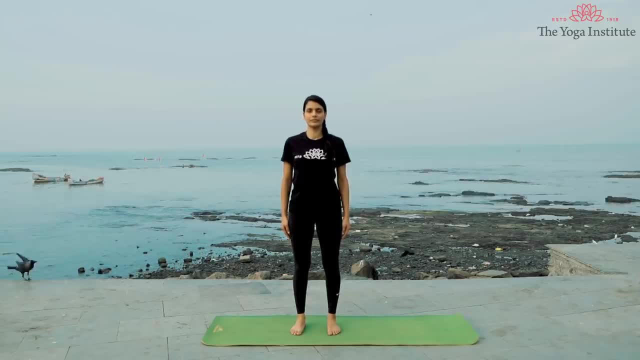 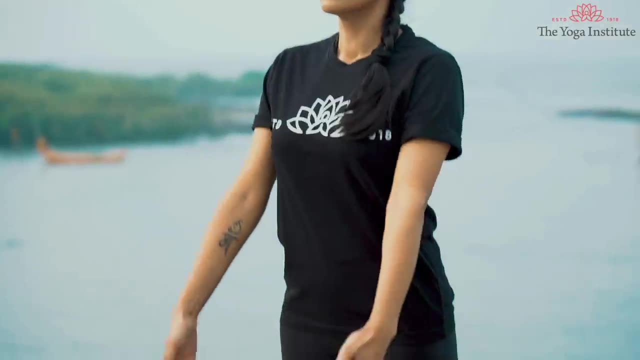 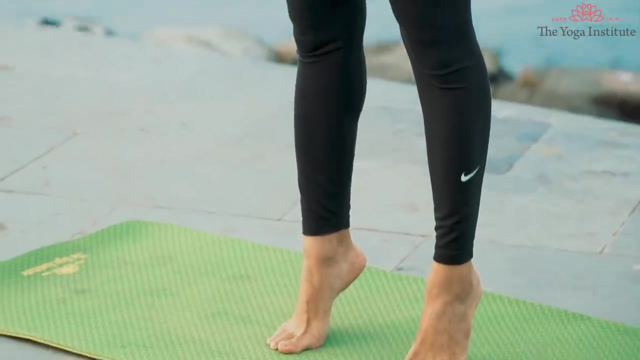 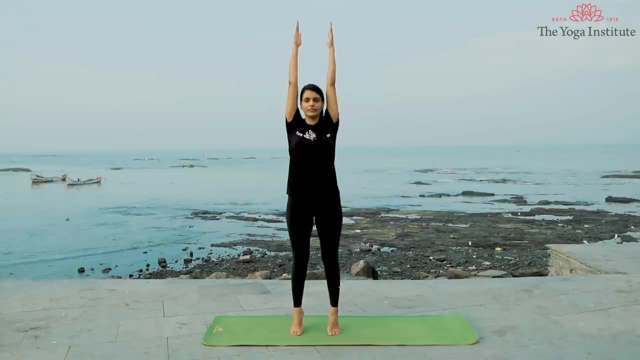 This is your starting position. Now raise both your hands smoothly above the head, Taking your hands for three seconds, and go up onto your toes simultaneously. Hold your posture here for a few seconds. Hands and fingers are stretching upward. Keep your hands close to your ears, both palms facing inward. 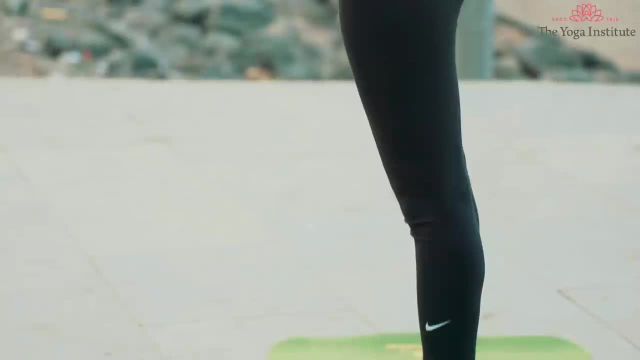 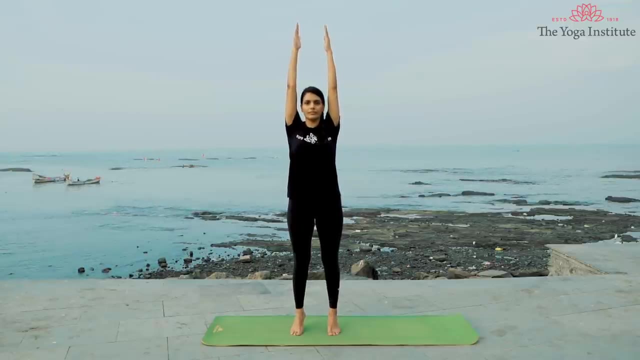 Breathe in and breathe out comfortably, Naturally Now, feeling this nice stretch in your calf muscles, focus at one point in front of you. Feel the weight on your toes. If your body tends to sway, try to stabilize your posture here. 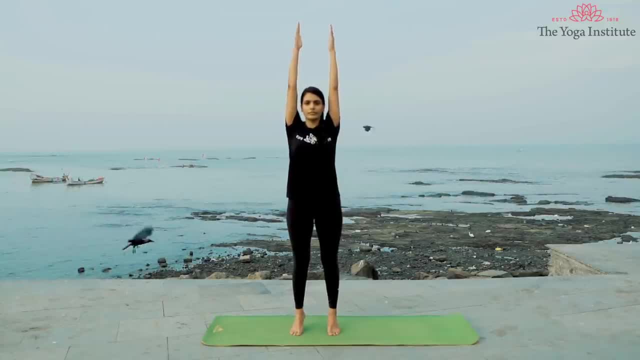 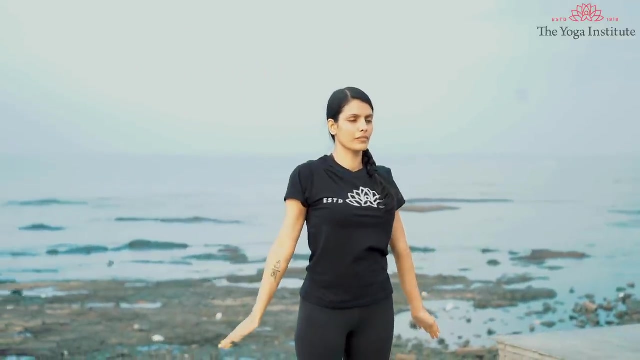 Keep stretching your body up as if you're stretching to reach the sky. This gives a nice elongation to the spine. Slowly exhaling out, bring your hands back to the side of the body, Synchronizing these movements together: Hands and toes. 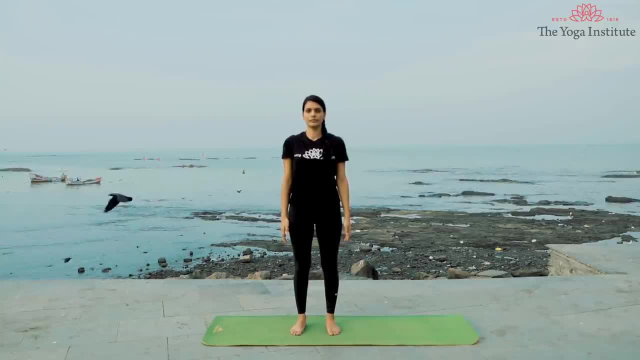 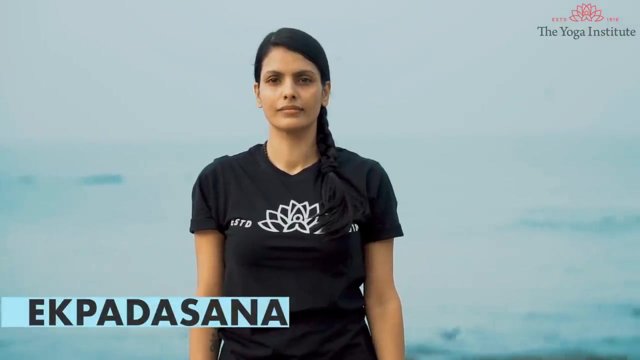 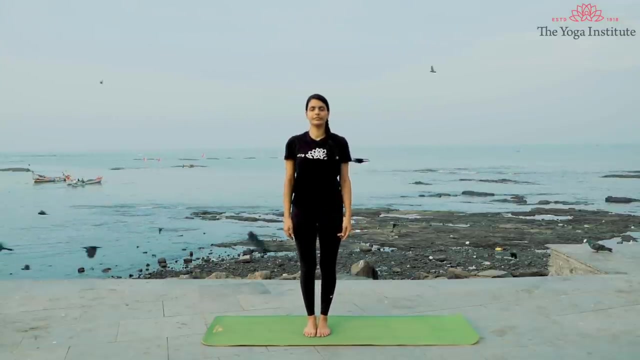 Synchronized Rest back onto your heels. This asana gives a nice stretch to your entire body. You really feel opened out. Now let's move on to Ekpadasana Balancing pose. Keep your feet together, Stand erect, with your eyes fixed at one point in front of you. 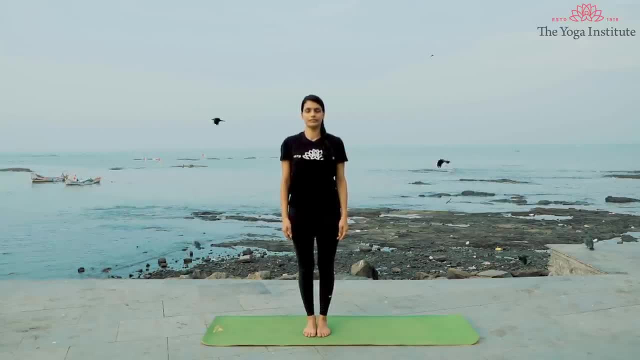 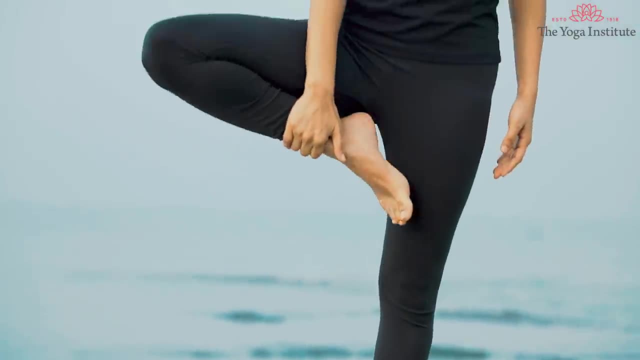 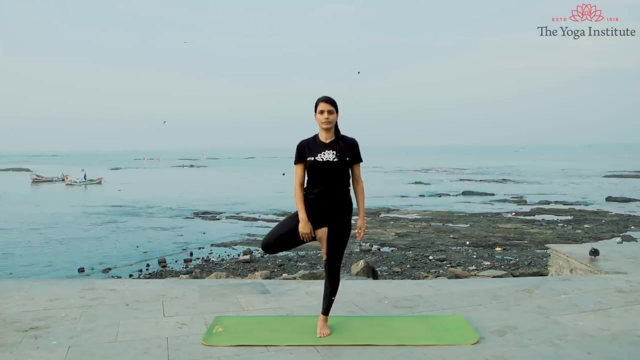 The fixing of your gaze is very important for this asana. To maintain the balance, lift your right leg up and place it on the inner thigh, bringing the weight on to your left leg. Now join your palms in Namaste, at the center of the chest. 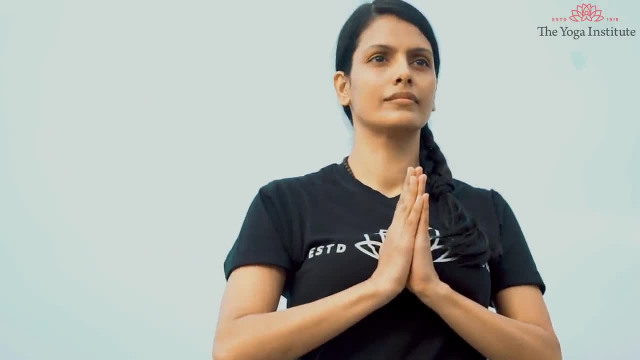 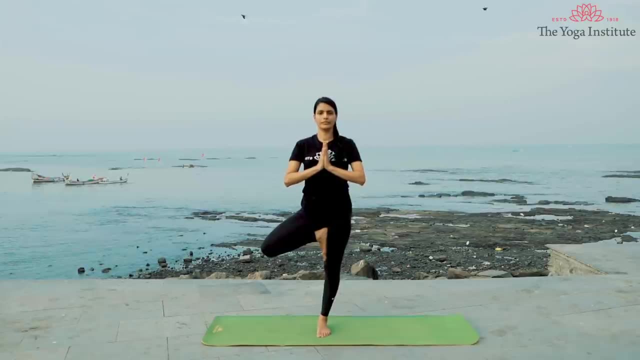 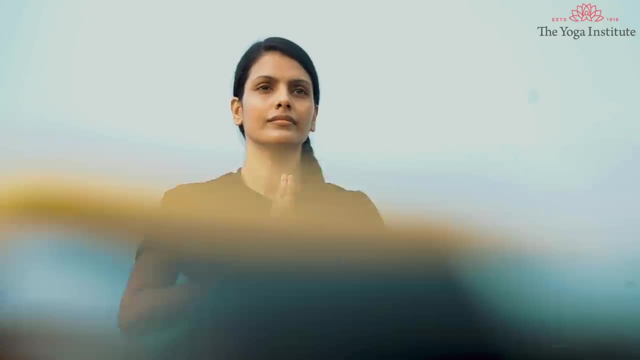 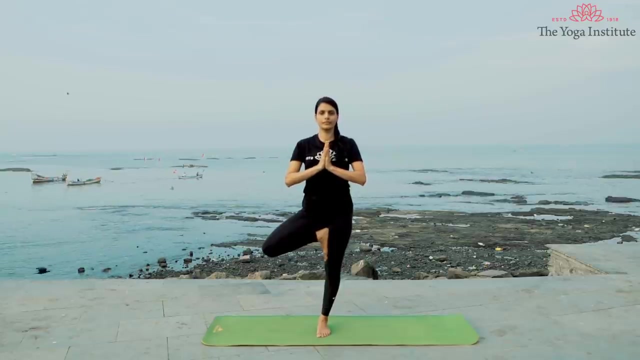 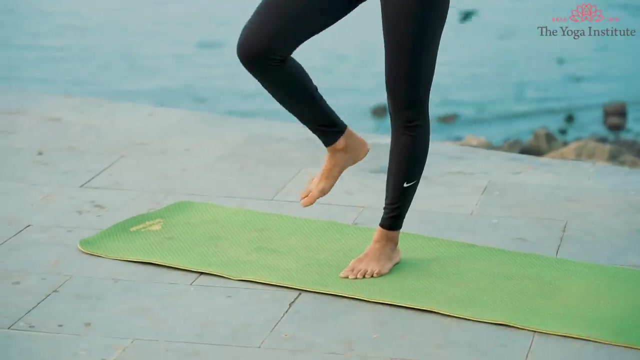 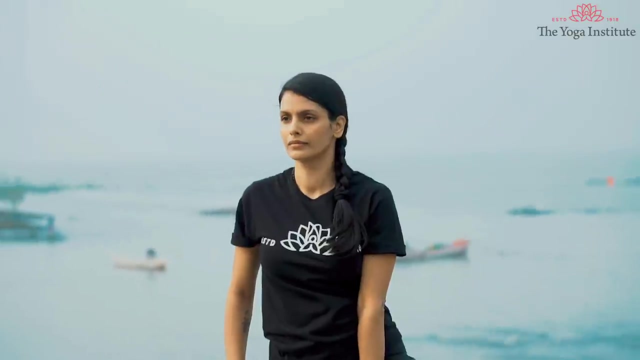 Stay steady and focused. This asana enhances our mind's ability to concentrate. Slowly bring your feet down and repeat the same thing with the other leg. Raise the left leg up and place it on the center of the chest. Place it onto the inner thigh of the right leg. 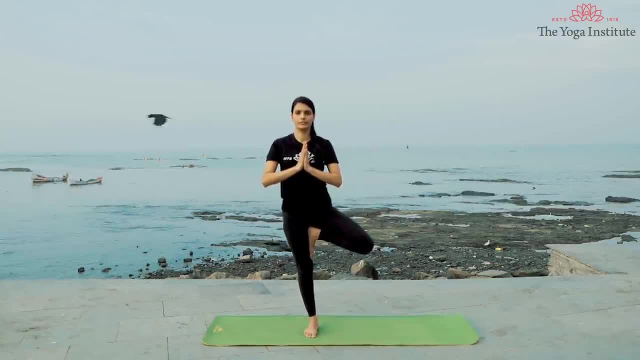 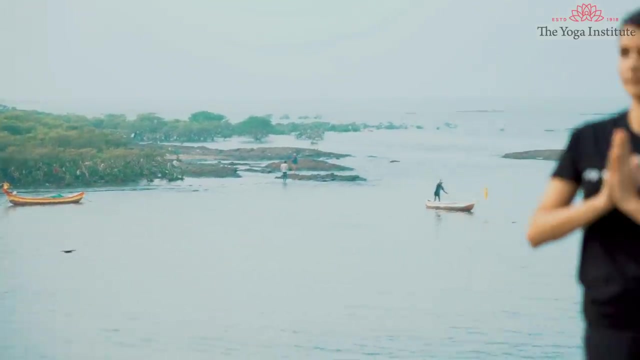 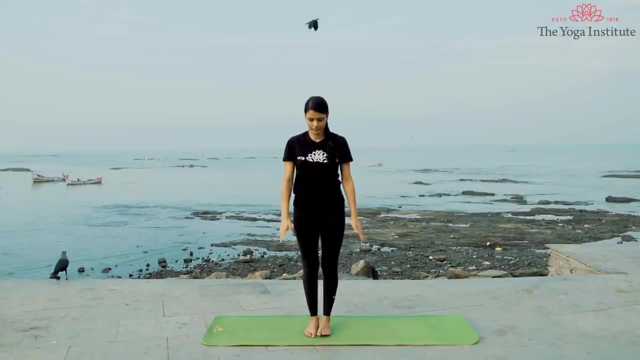 Find your balance. keep your gaze steady. If you need to, you may count 10 backwards mentally to keep the mind engaged. Keep your spine erect, feel the firmness under your feet And now relax both your feet back to the initial position. 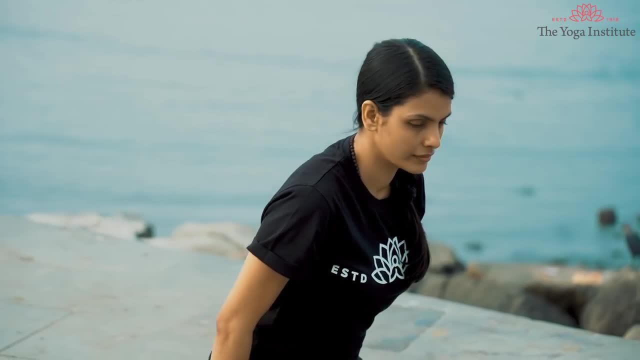 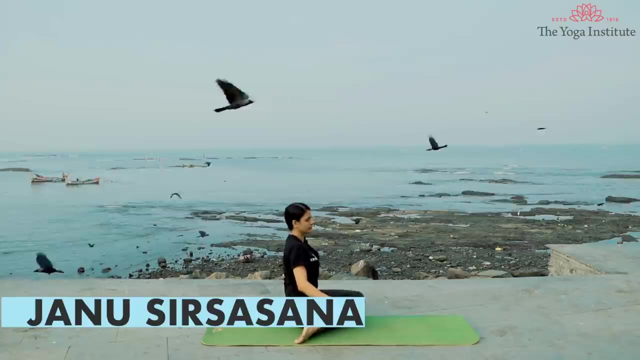 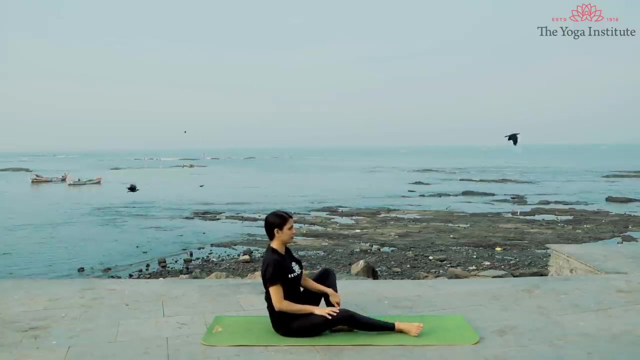 Slowly sit down in Vajrasana. Slowly stretch your legs out for Janu Shishasana. Sit in a comfortable cross-legged position. Take your right leg forward Straight And left foot placed onto your inner thigh, Knees comfortably placed on the ground. 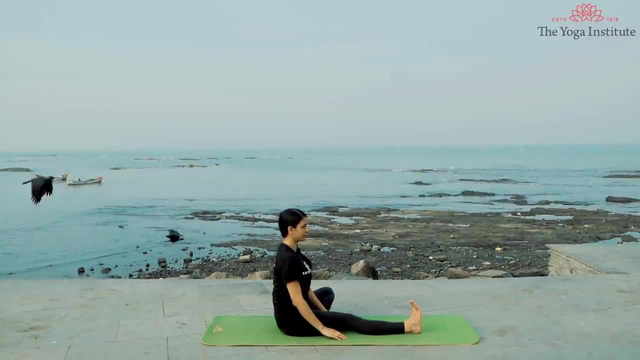 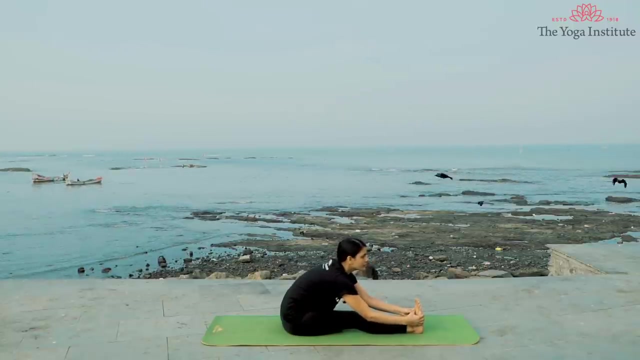 Sit erect. The lower back might tend to slouch, but try to lift it and keep your spine erect. Now, inhaling, raise your hands up and, exhaling, bend forward to grab the foot or grab your ankle. If you're unable to touch your toes or your ankle, that's perfectly fine. 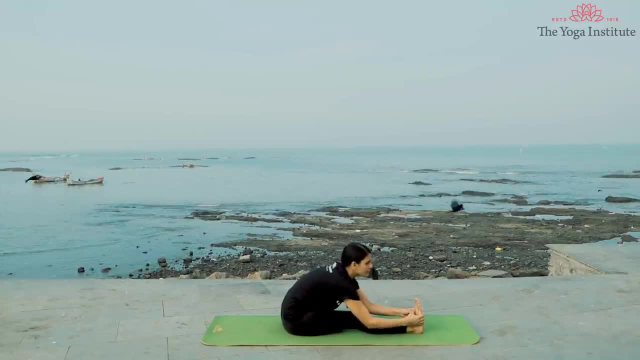 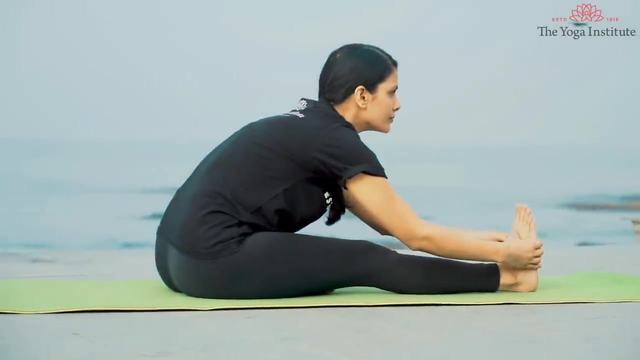 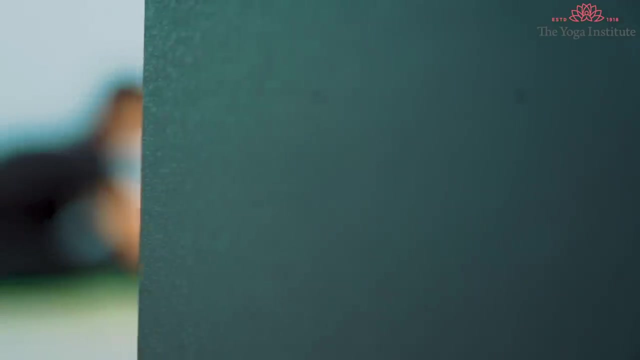 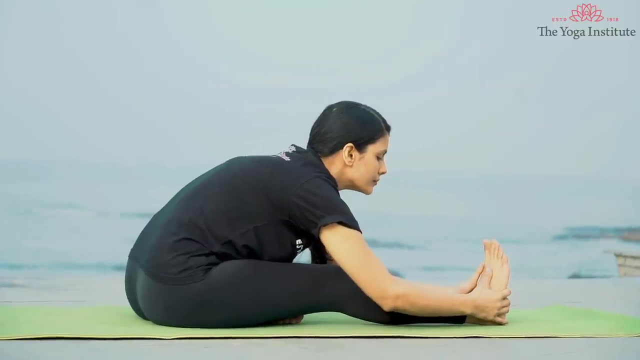 Move to your capacity. The thighs might tend to lift up, but try to press them down firmly on the ground, Exhaling further. bend and catch your toes. Try to keep your spine straight. Lengthened rather Good, Feel the stretch in your hamstrings and calf muscles, keeping your elbows bent. 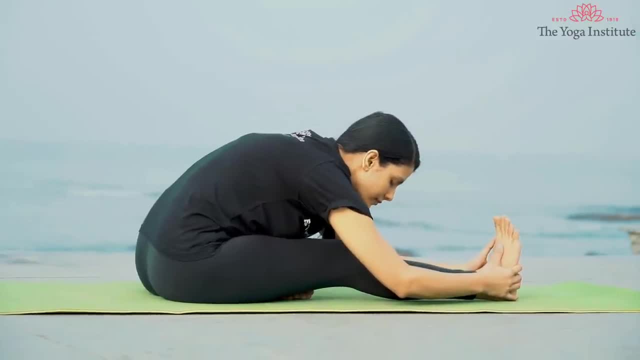 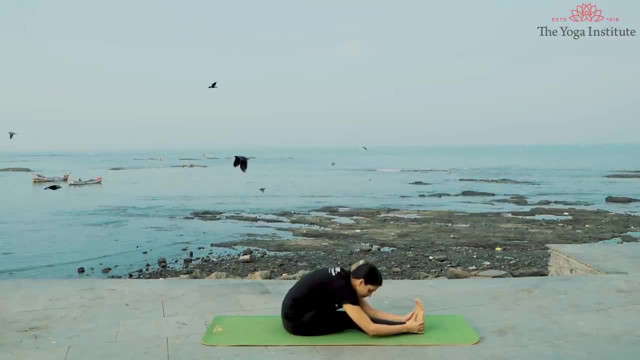 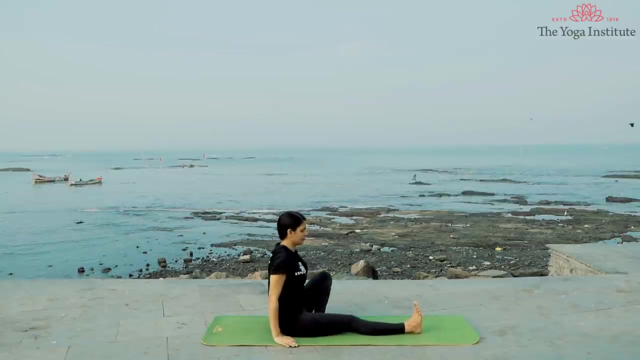 Try to drop your body to gravity. Let go your body down. This shall help you go down further Inhaling. come out of the position And let's repeat this on the other side. Stretch your left leg out And place the right foot. 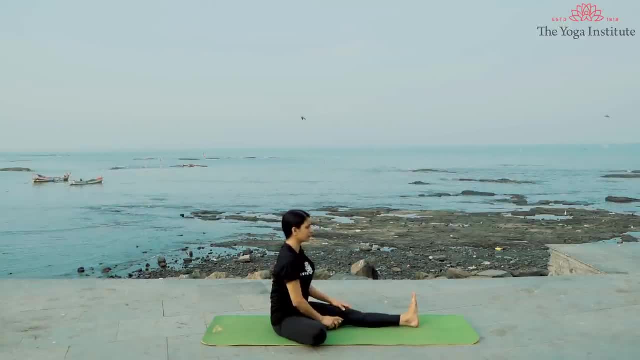 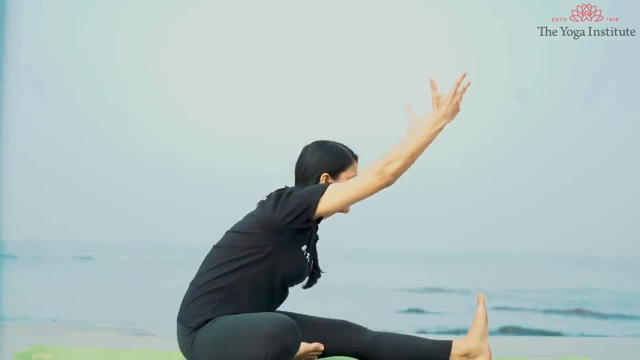 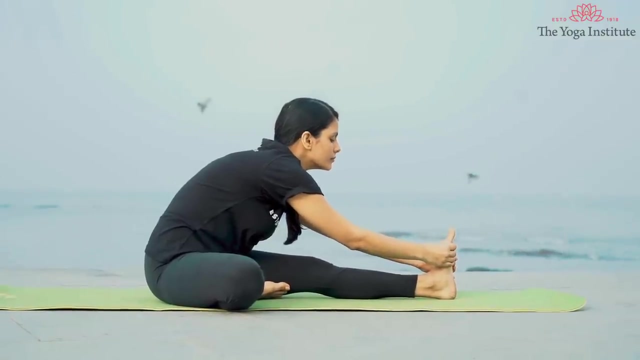 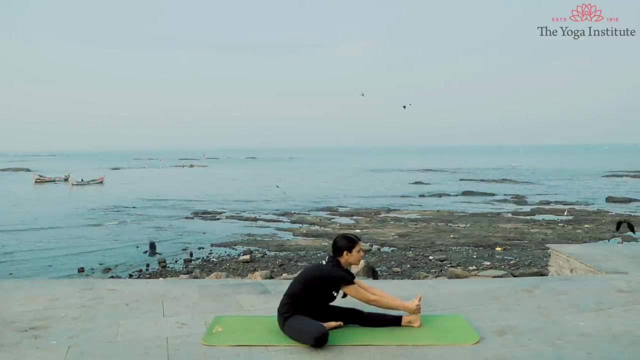 And place the left foot onto the thigh of the left leg. Stretch your arms, Inhale here, Lengthen the spine And, exhaling, reach forward to grab the big toe of the stretched leg, the left leg. If you can't reach your toes, you can always grab your ankle or shin. 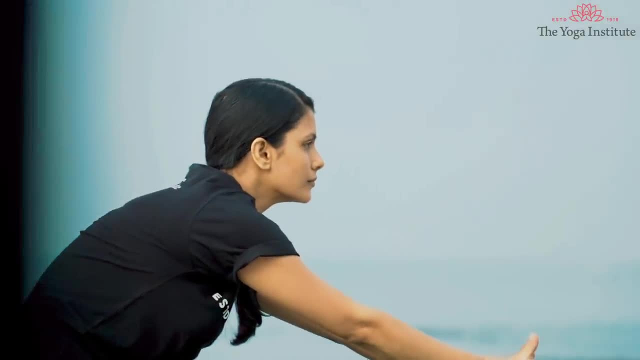 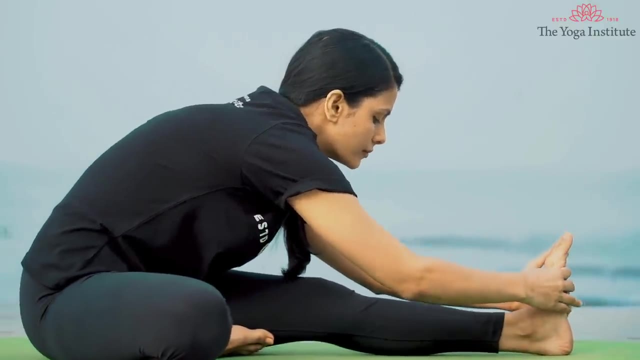 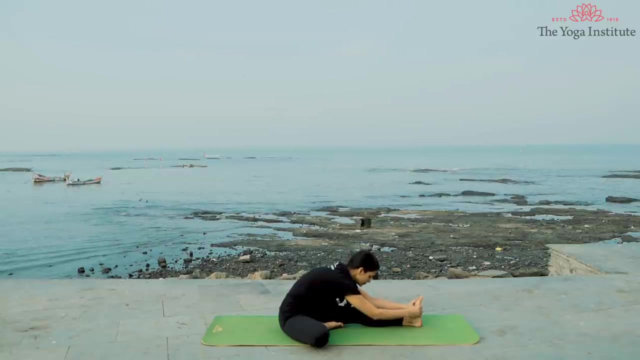 This asana is very effective and it is done with the attitude of surrenderance. Humility plays a huge role in forward bends. One progresses more when one is humble, Unless one has severe spinal problems. everyone can practice Janusha Shasana. 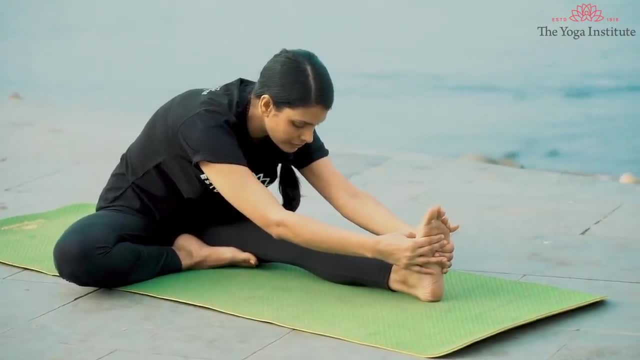 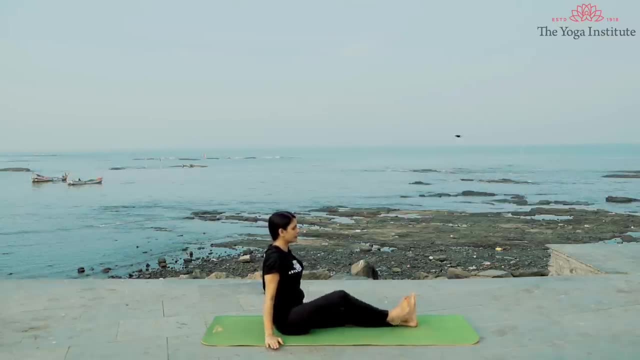 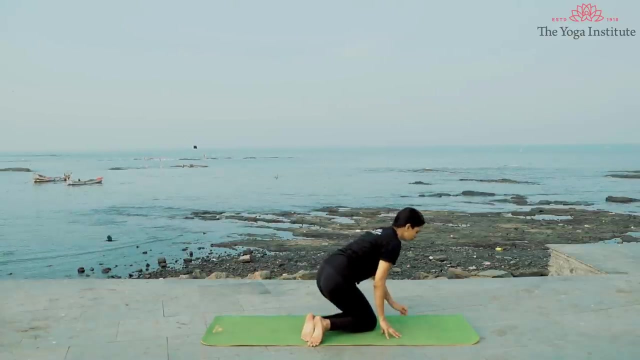 Inhaling, come out of the position, stretch your arms up and exhaling, relax. Let's get on to our knees for Marjariyasana Cat-Cow, Bring your hands and knees in table pose with a neutral spine. 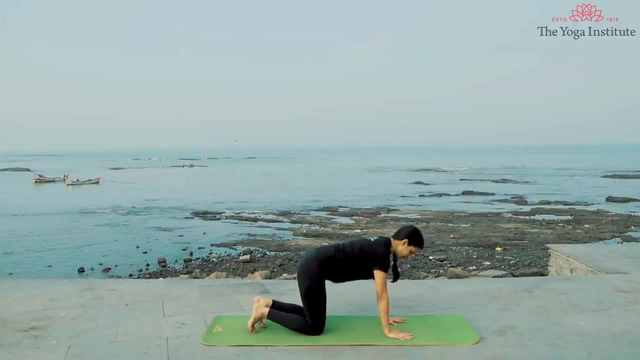 Hands firmly placed on the ground and at shoulder level distance. Your thighs in line with the hips. Hands firmly placed on the ground and at shoulder level distance. Hands and legs perpendicular to your upper body. Now, as you inhale and move into cow pose, lift your sit bones upwards. 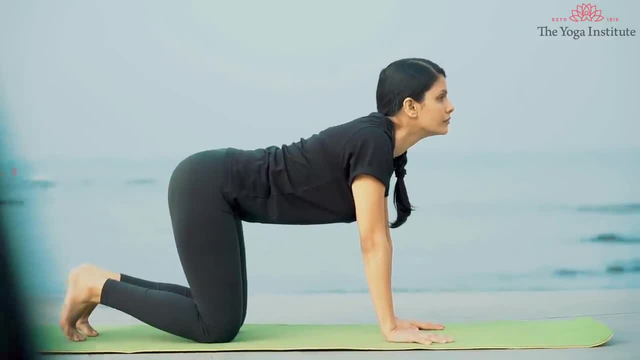 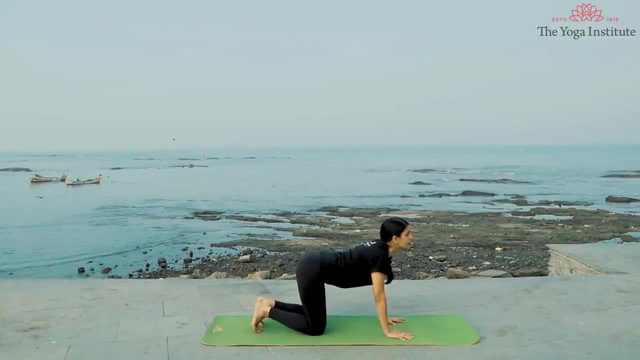 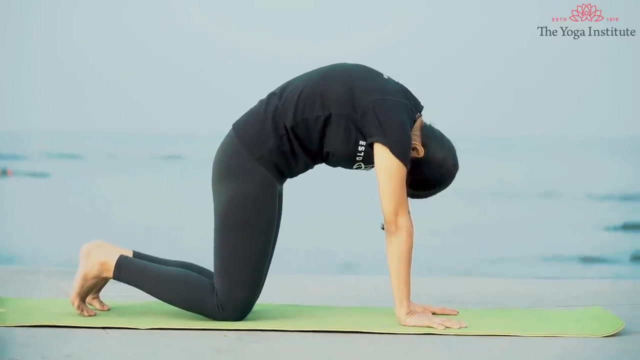 Press your chest forward and allow your belly to sink. Lift your head, relax your shoulders away from the ears and gaze straight ahead As you exhale. come into the cat pose while rounding your spine outward, Tucking in, Tucking in your tail bone and drawing your pubic bone forward. release your head towards the floor. 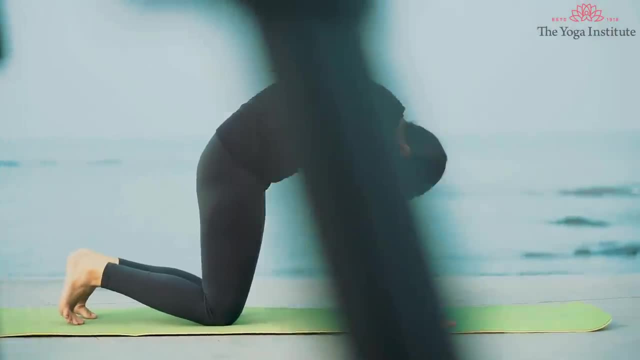 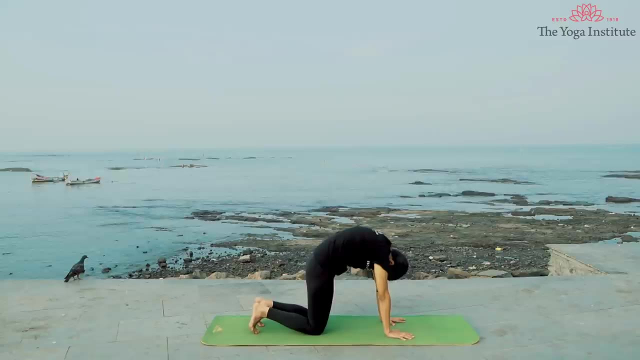 Just don't force your chin to your chest. Most importantly, just relax. In case of knee pain, avoid resting onto your knees or place a pillow underneath your knees. You may even double fold your mat Now slowly come back Sitting onto the body. 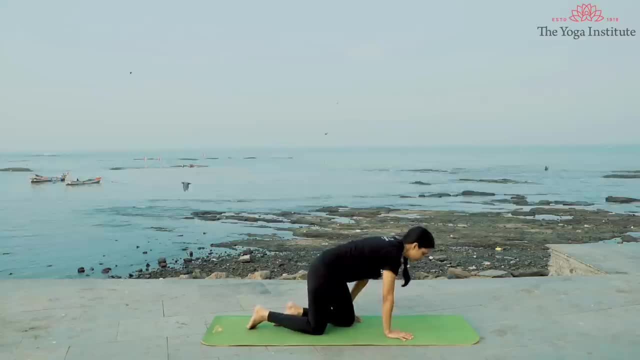 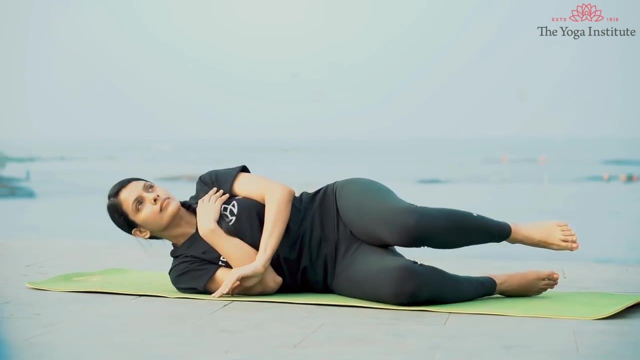 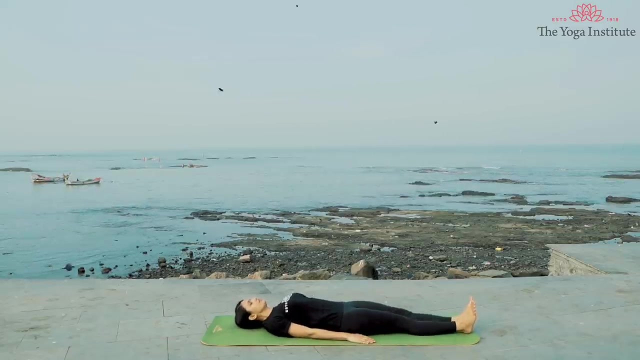 Slowly turn to one side, lie down onto your back for pavanmukthasana. We'll start with the one leg variation Where you lie down. adjust your lower back by sliding your hips and tail bone down towards your heels. 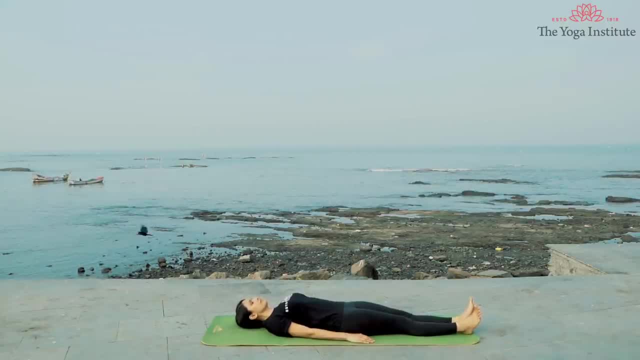 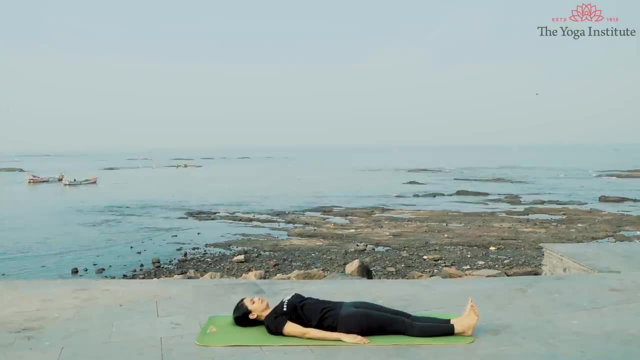 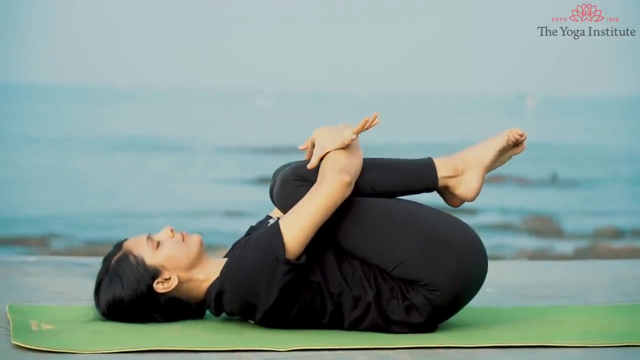 So that the lower back is firmly resting on the floor without an over arch. Staying on your back, take a deep breath And, as you exhale, bring both your knees towards your chest and press them towards the abdomen. Clasp your hands around your legs as if you're hugging your knees. 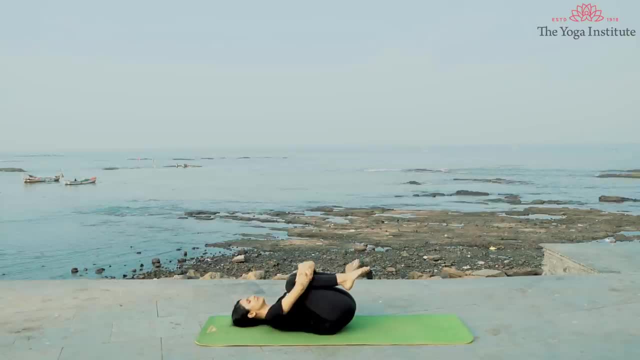 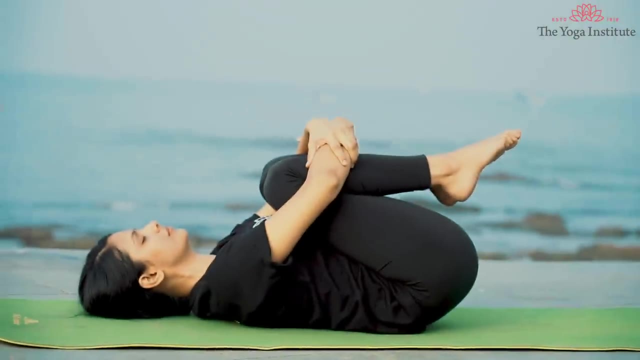 Hold this asana while you breathe normally. Every time you exhale, make sure you tighten the grip of your hands on the upper shins and increase the pressure on your chest, And, as you exhale, bring both your knees towards your chest and press them towards the abdomen. 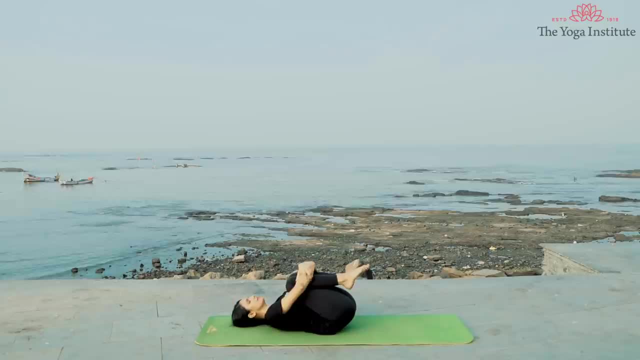 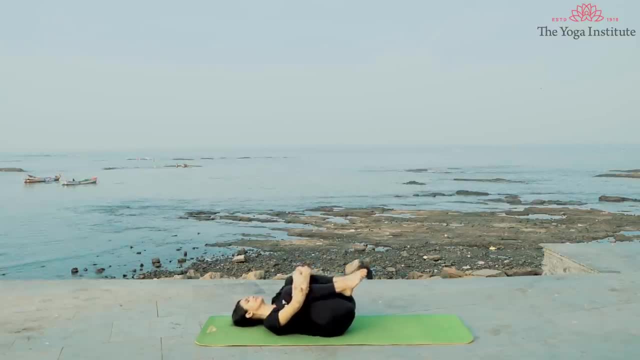 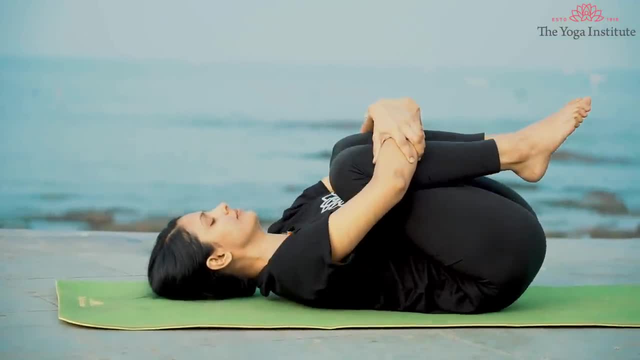 Exhale and release the pose after you rock from side to side about three to five times After that stretch. After that stretch, And finally, the pose for relaxing the entire spine and body- yastikasana. And finally, the pose for relaxing the entire spine and body- yastikasana. 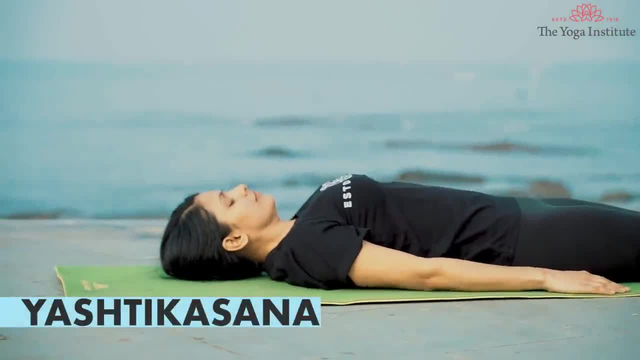 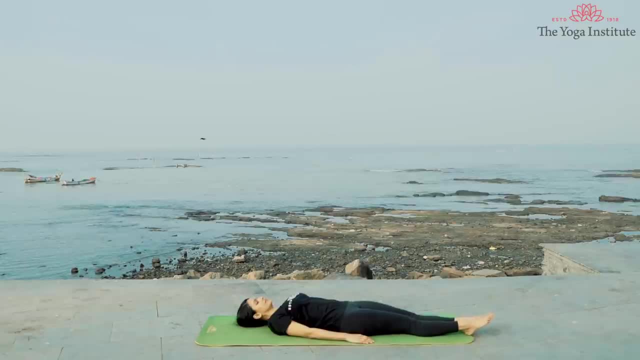 And, finally, the pose for relaxing the entire spine and body: yastikasana, relaxing the entire spine and body. yasthikasana, stretch your legs out, rest your hands at the side of the body and inhaling. extend your arms above the head. 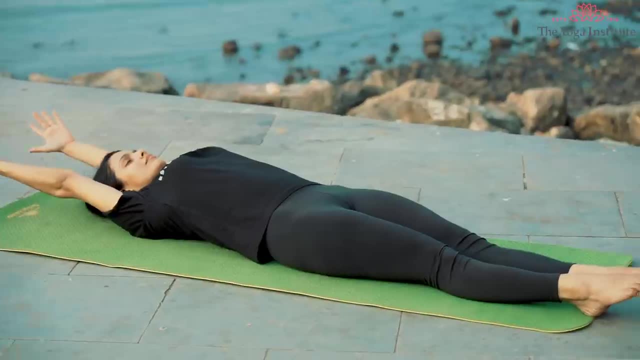 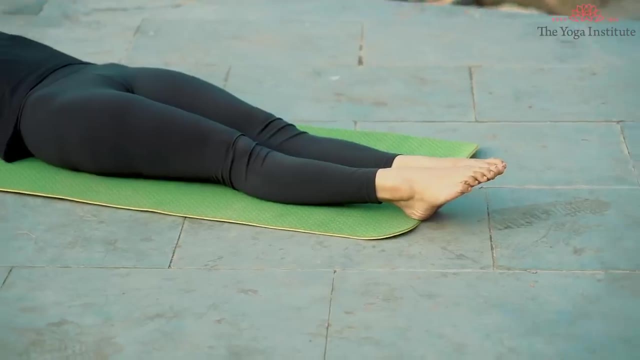 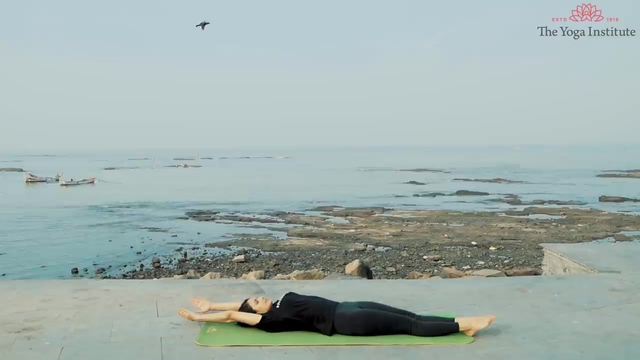 stretch your feet, stretch your toes, stretch your hands in opposite directions. visualize your body to be a piece of stick being stretched on both ends, allowing the spine to really lengthen and de-stress, exhaling. come back, rest your hands back at the side of the body and now, slowly, 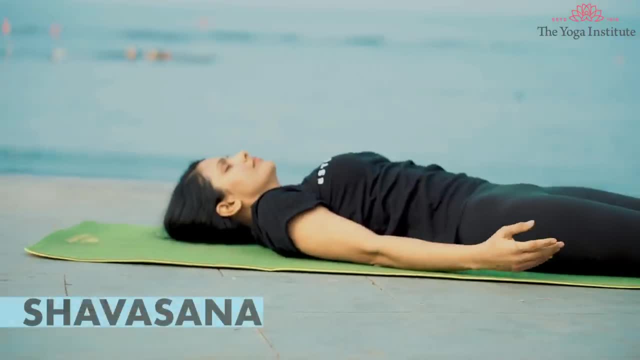 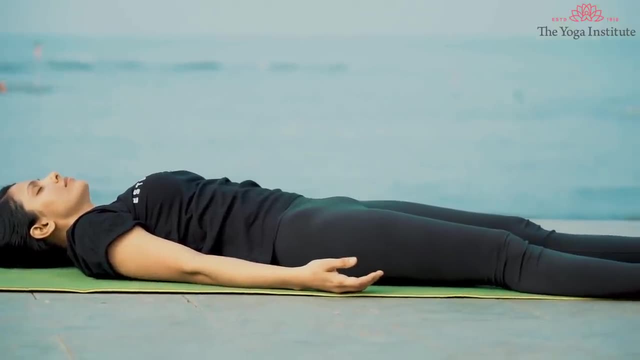 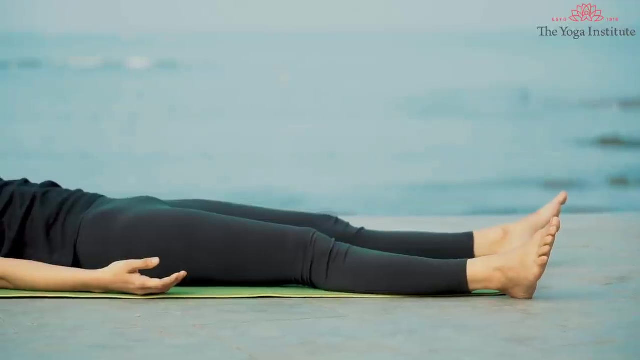 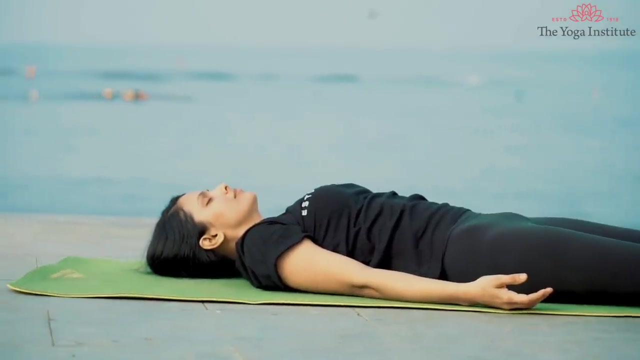 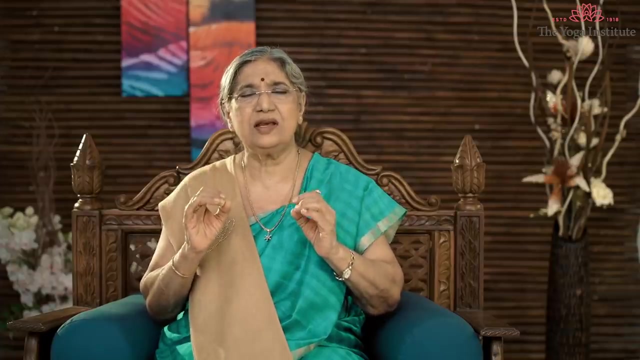 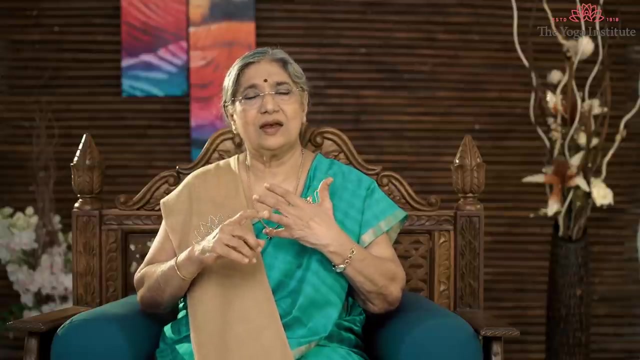 get into shavasana, separate your legs, separate your hands, allow complete, deep relaxation. or to suggest yourself i'm letting go and relaxing completely. namaskar, every human is different. every human is a unique personality. every human has his own body, his own mind and his soul, soul, universal. 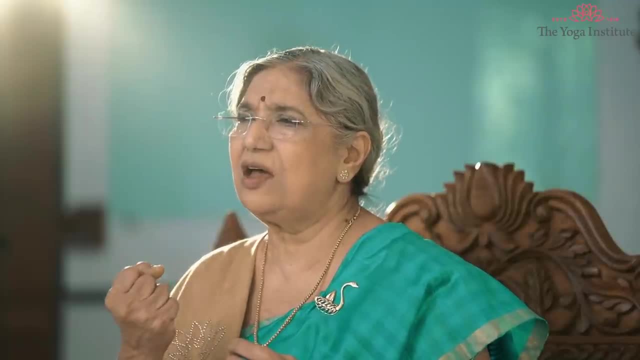 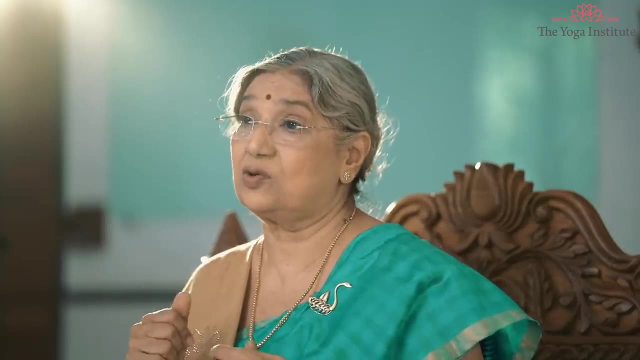 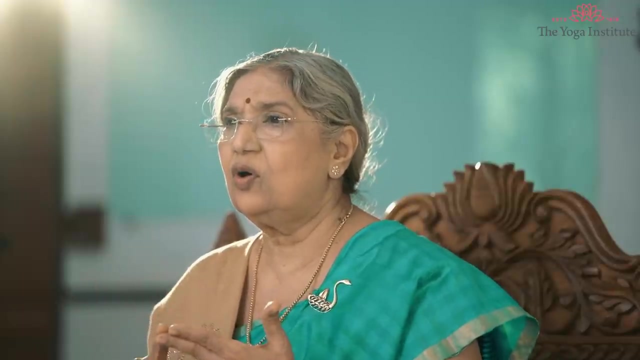 it is consciousness that means we have divinity within us and we are all potentially divine. but body and mind has to be understood. we have a duty to understand our own body and our own mind. so to understand that certain asanas are very important, all of us should. 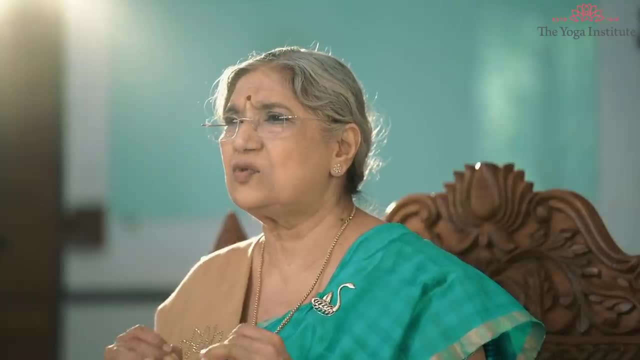 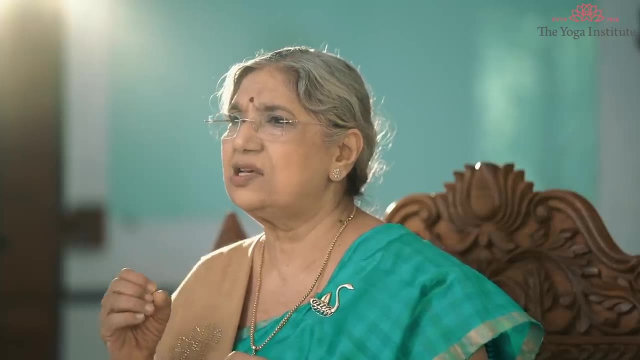 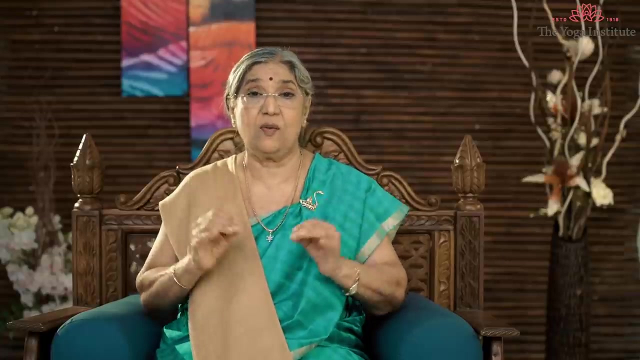 know that when we do our asanas- any part in our body, if it is weak, that would come to the surface. weakness would be understood And the moment you understand the weakness you can do something about it and strengthen it and help yourself. So, with such awareness about doing asanas, 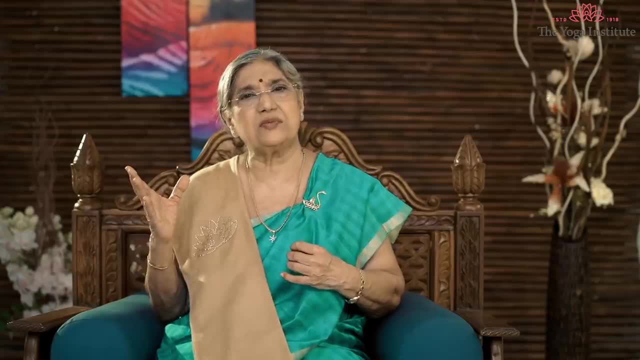 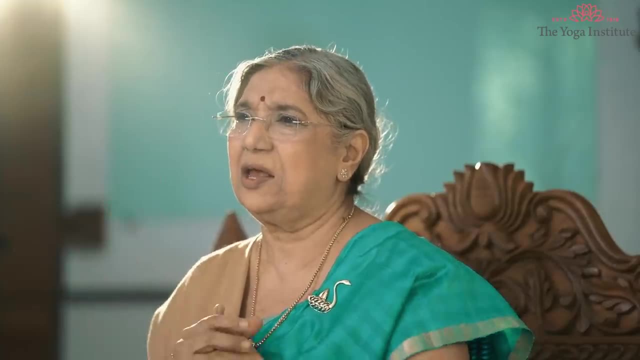 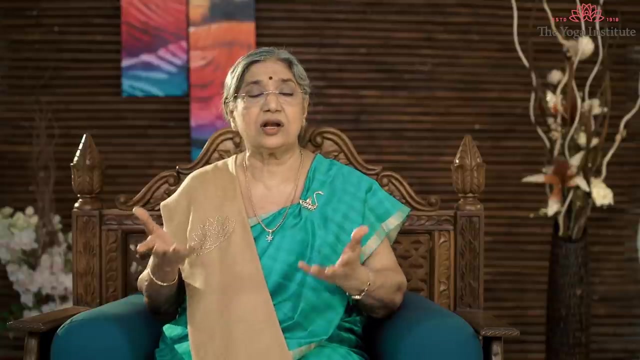 and knowing your weakness, you prevent major problems of your life. Diseases will never set in if you know how to catch the disease right at the beginning. Similarly, mind that human mind, when it gets disturbed, you sometimes don't even know that you are under tension. 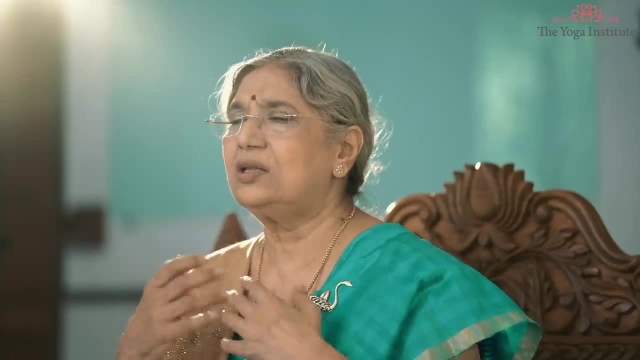 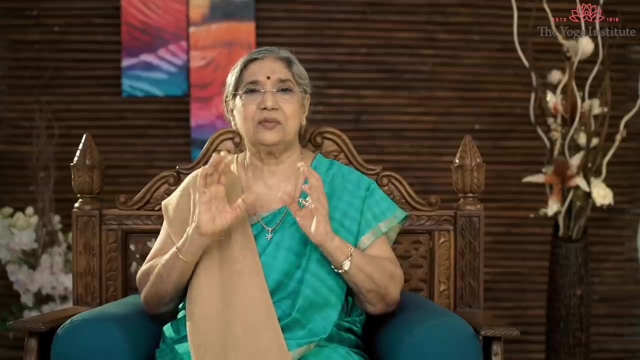 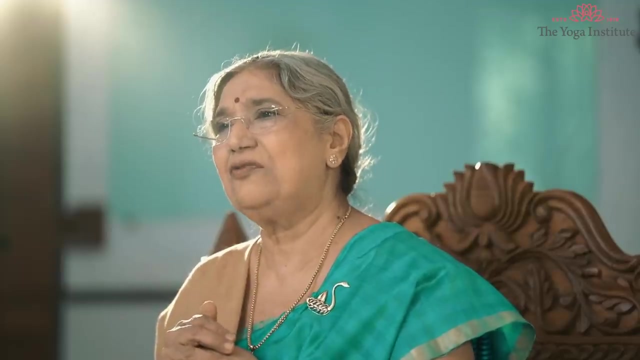 and disturbed. but you watch your breath and you will come to know that you are disturbed. So make your breath under control, bring it smooth, bring it systematic and you will remove your tension. So this is how we are supposed to manage our life and help ourselves: by knowing.